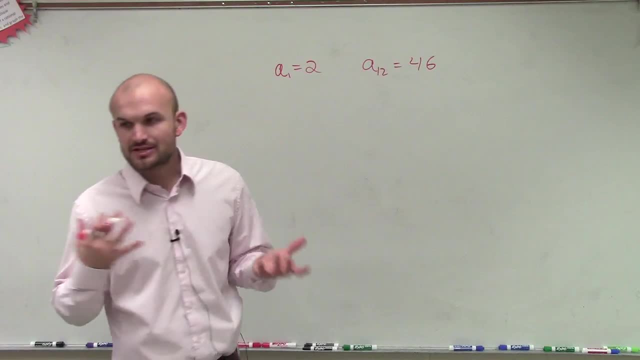 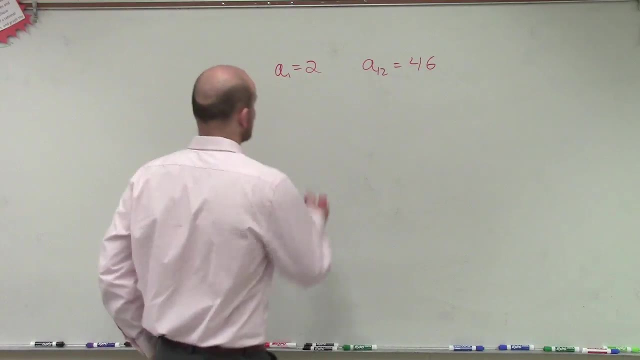 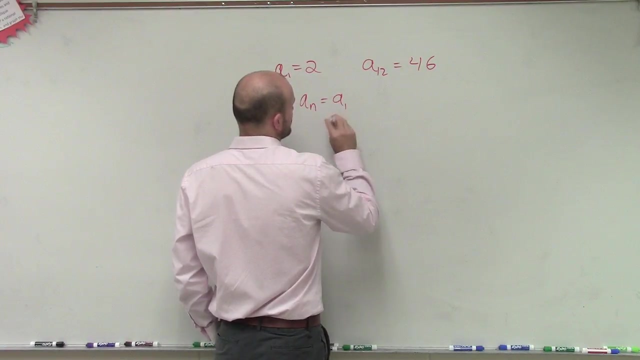 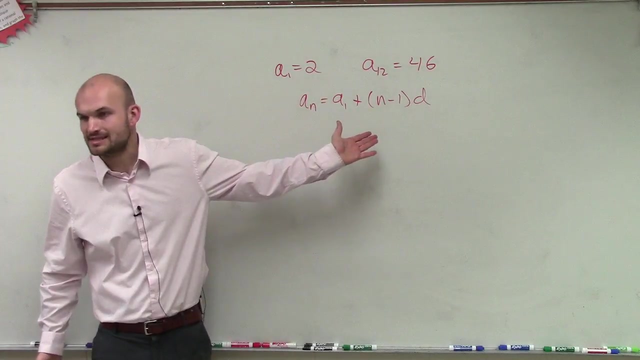 Okay, so remember our famous formula that we have. I gave you guys two formulas: one for the nth term of an arithmetic sequence and two for the sum. So the nth term stated that if I had a sub n equals a sub 1 plus n minus 1 times d. Now this is obviously to be used when we had a sub 1 and to be able to find a sub n when we knew what d was. 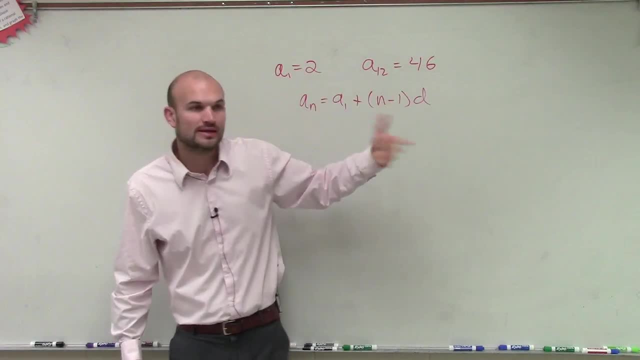 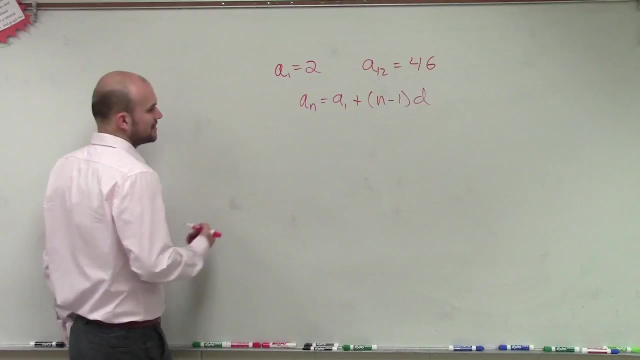 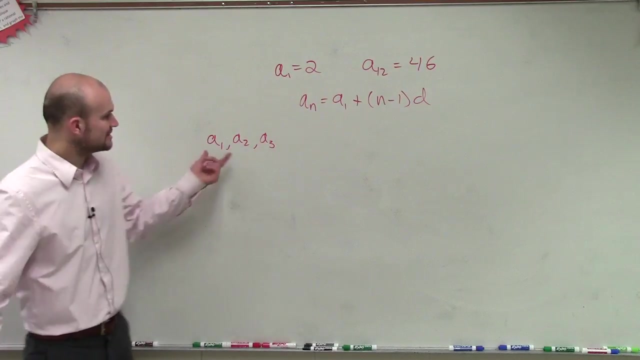 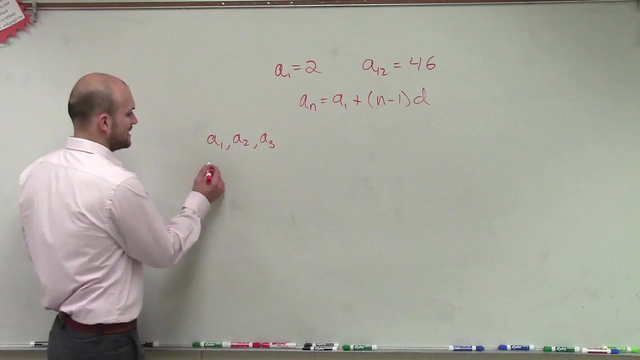 However, when given these two terms, we don't know what d is. So we need to find the value of d. Does that make sense? Okay? so let me go and take a look at. let me give you an example. If you guys remember arithmetic sequence, is the difference right between a sub 1 to a sub 2 and a sub 2 to a sub 3, right? Yes, So what we'd say is: you know, a sub 2 minus a sub 1 is equal to a sub 3 minus a sub 2, correct? 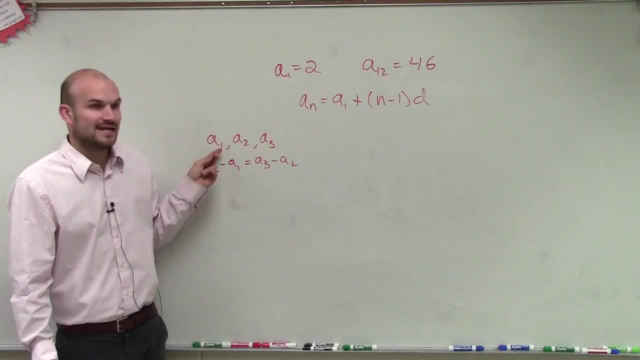 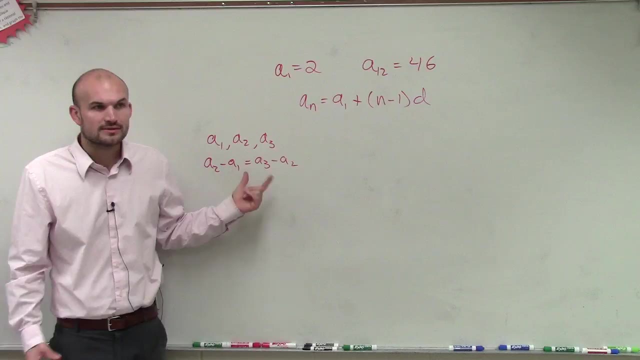 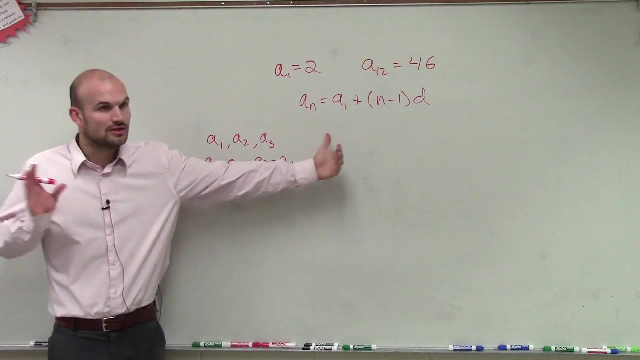 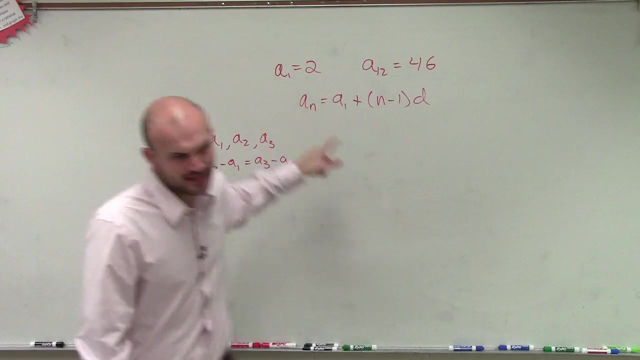 However, could I take a sub 3 minus 1 and then divide that by 2, and would that still give me the difference? Yes, I mean, they're still going to have a constant difference, but if I don't have two consecutive terms, what I can do is I can still subtract them and but be able to find what the difference is. So what I'm saying is: I don't have this is an a sub 1, was it a sub 1?? Okay, they do give us a sub 1.. All right, So they give us actually a sub 1.. So that's okay. 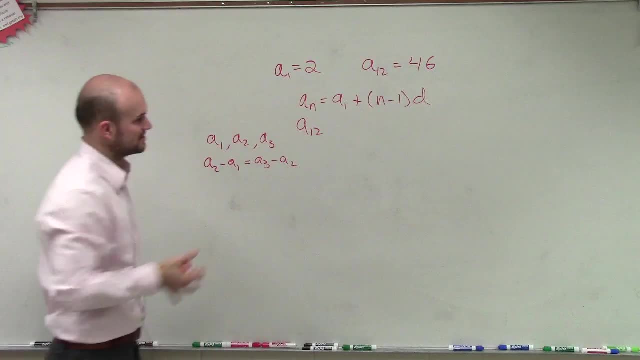 So we have a sub 12,. therefore, that thing I was just talking about is not really going to apply here. So we want to figure out what a sub 12 is. equals a sub 1, which we now know is 2.. 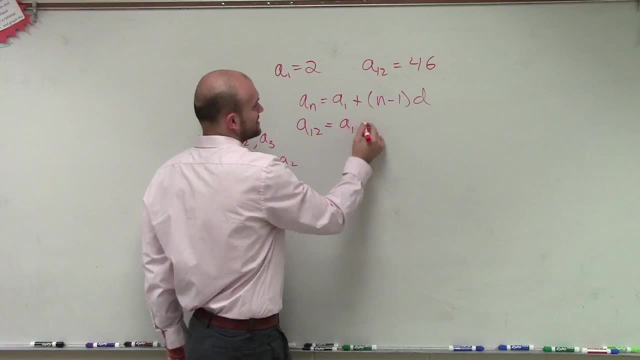 Oh sorry. so a sub- no, it's just right in here a sub 1 plus now, since I'm finding out a sub 12, that's going to be my n is 12 minus 1 times d. 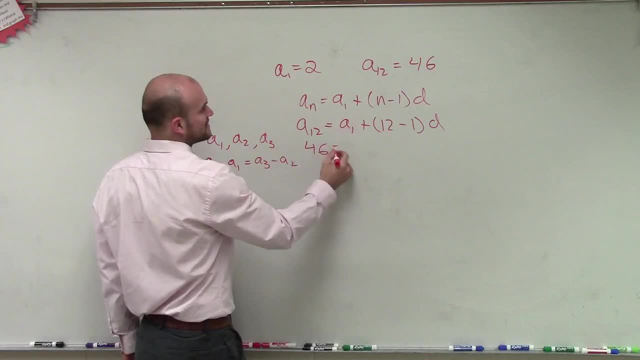 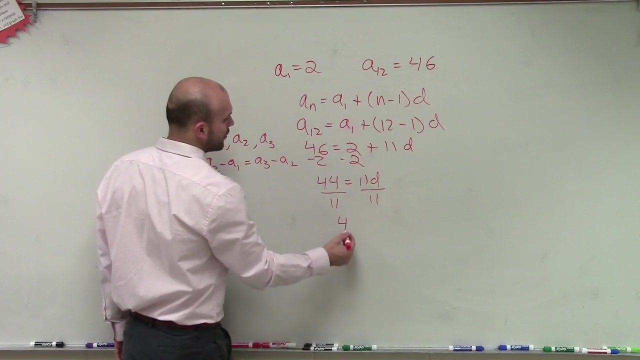 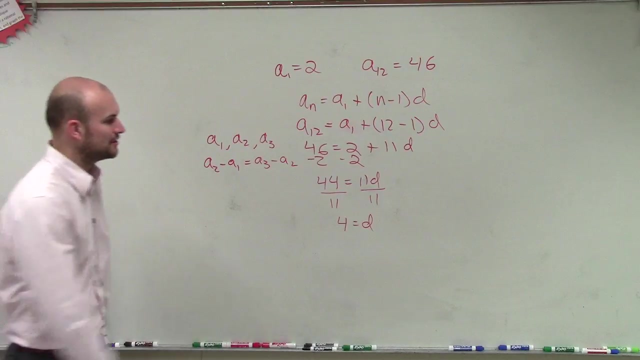 So a sub 12 was 46 equals 2 plus 11d minus 2.. 44 equals 11d. divide by 11, and you could say 4 equals d And then. so now you know that the difference is 4, so if a sub 1 equals 2,,